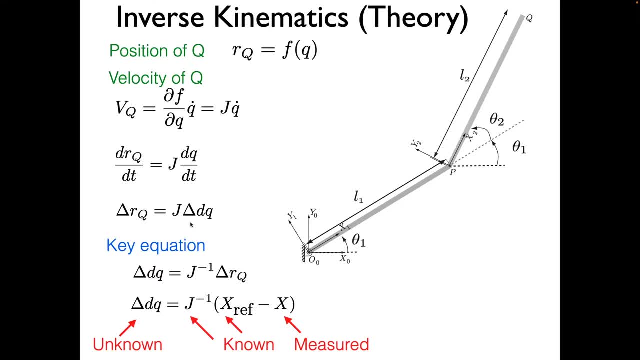 We can cancel dt and we are left with drq equals j delta q. The key equation is actually this equation: If we invert j we have, we can solve for dq. It is j inverse delta r. So what we do here is in the numerical method. I'll show you delta. rq is the 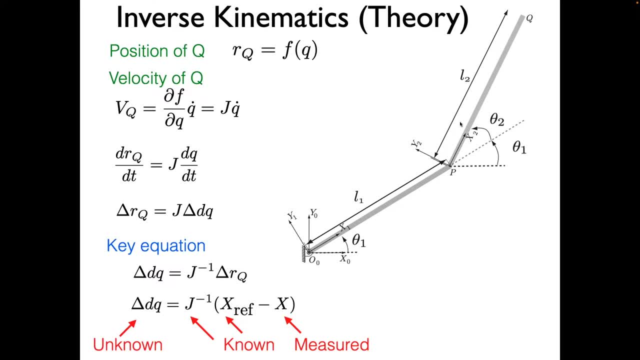 difference between the reference minus delta rq and the difference between the reference minus delta rq. So this is the reference minus the measured position of the end vector. So remember, the position would be x and y coordinates. that is embedded here. j, in this case, would be: 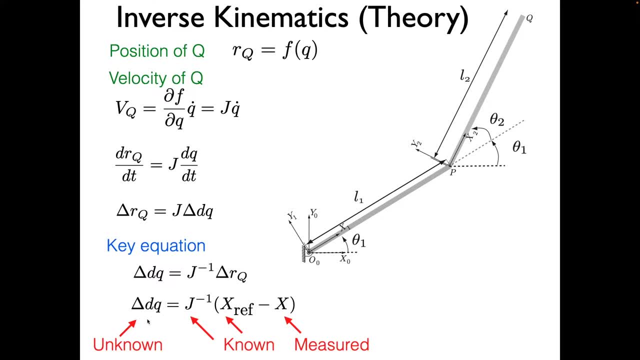 2 cross 2, so it will be the inverse also will be 2 cross 2, and that will give us the correction in q or correction in theta, which you then need to add to theta 1 and theta 2 in order to compute. what is the change we need to do on theta 1, theta 2, so that q can draw whatever curve you wanted to. 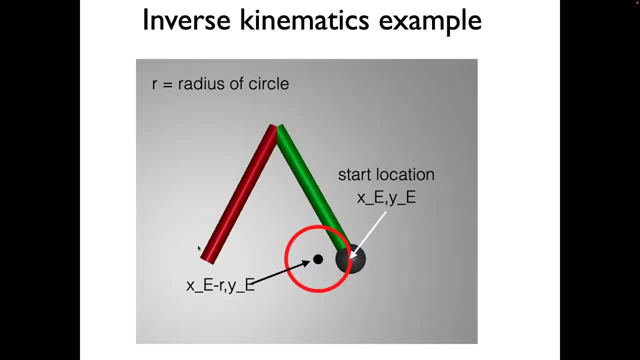 draw. In this case we will use MuJoCo. We will look at two link example. We will try to get the end effector to draw a circle. We will start the end effector at at one of the along the x-axis, like it's shown over here, and 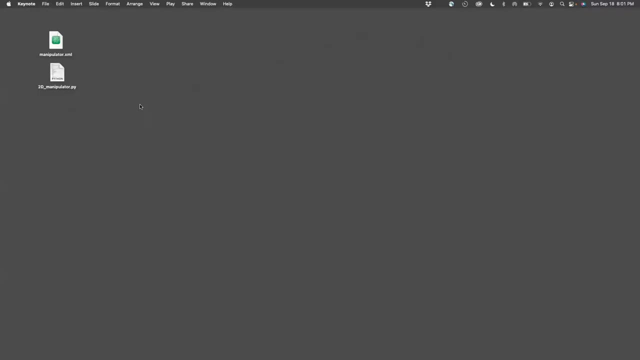 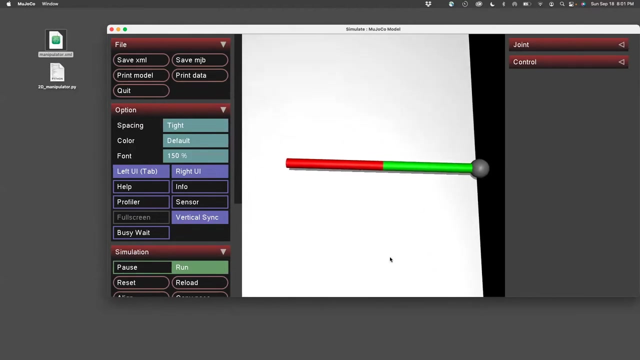 then we'll get it to trace. this curve Sample builds off the two link manipulator I had done earlier, so I'm going to open that in in the simulator. Okay, so the manipulator consists of 2 links, the the gray sphere. here is the end effector position. 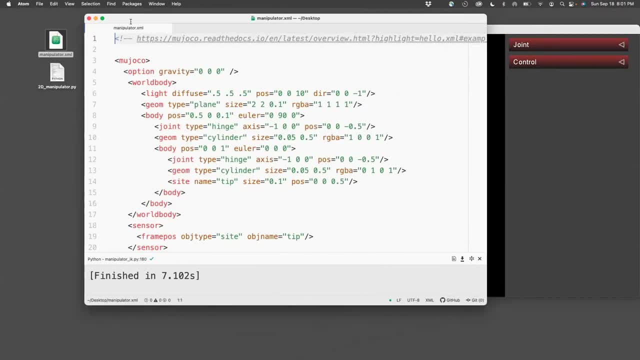 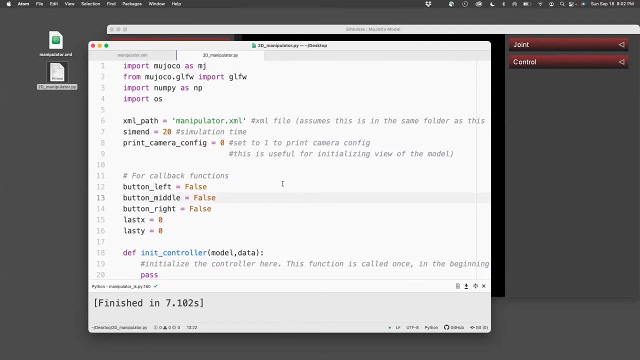 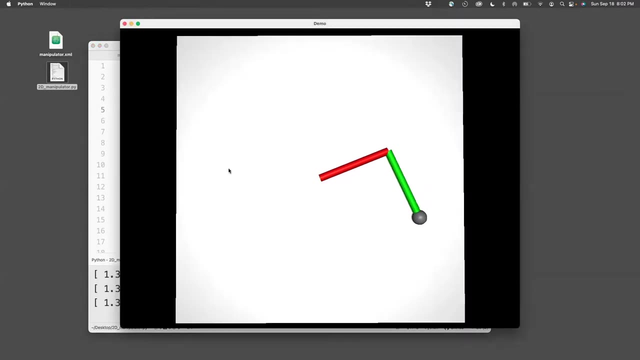 and this was modeled in this manipulator XML file 36 00 00 00. i also wrote a pie file which basically moves this manipulator in some fashion. So if I run this, then the works fine. the manipulator pretty much moves based on pre-specified angles: theta1 and theta2.. 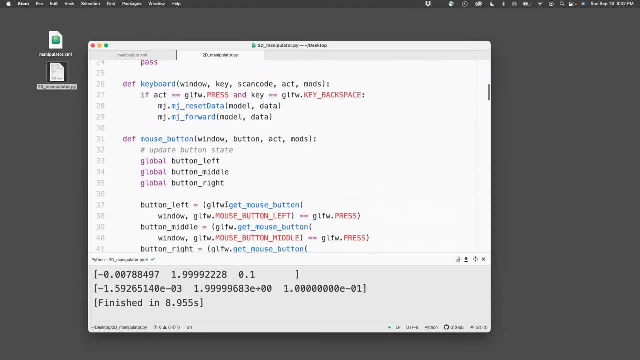 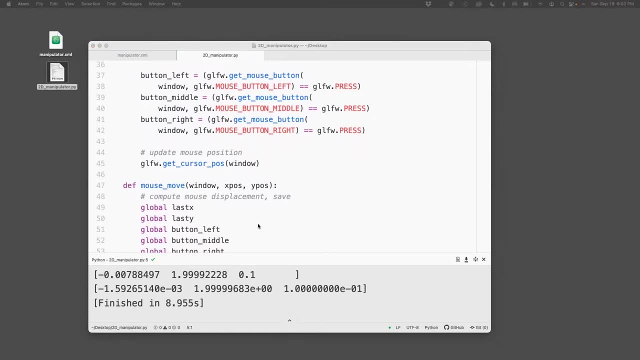 Okay, so we'll start modifying this. In this case, we will first fix a particular angle, and then we'll look how the animation looks, and from there we will go for the inverse kinematics. So what I'm going to do is I'm going to pretty much delete this code. 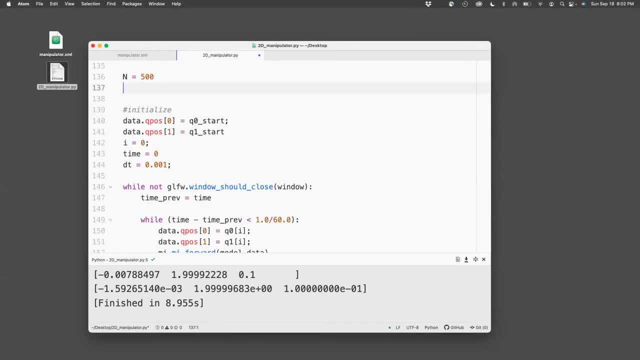 and specify my own angles for theta1 and theta2.. So I chose angles which work. Theta1 is pi by 3 and theta2 is minus n pi by 2.. These will be my initial angles, theta1, theta2, and if I want it to be, 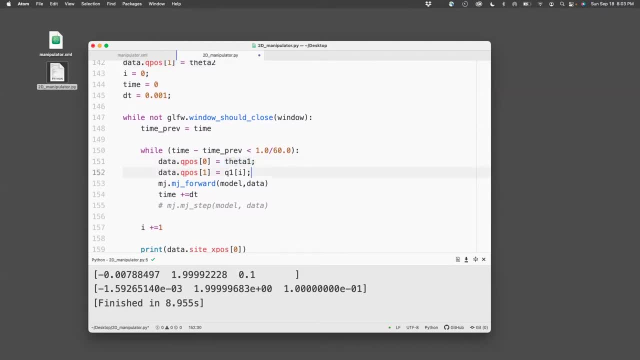 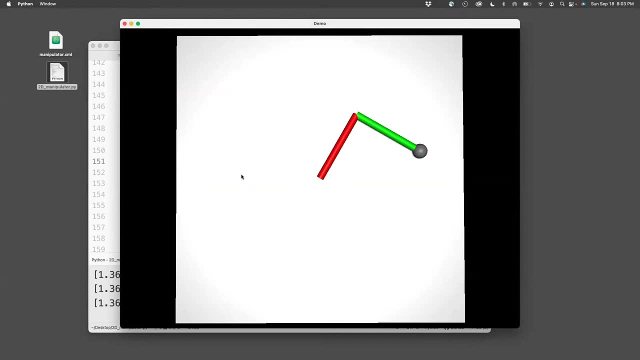 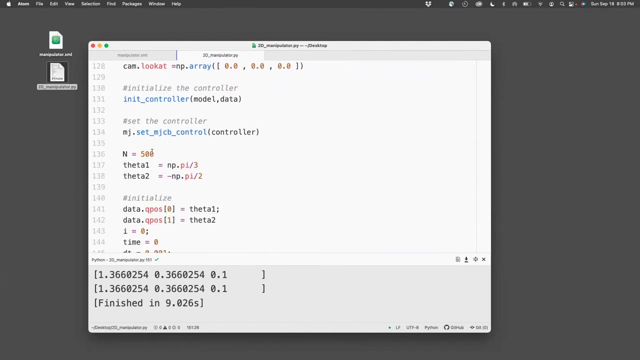 played in a loop which is specific one, so I'm going to run this and then you see that the manipulator is at particular position. Okay, so this stays a little bit long. If you want to shorten the time, what I do here is I'll change this n to, let's say, 100.. So the animation time will be short. 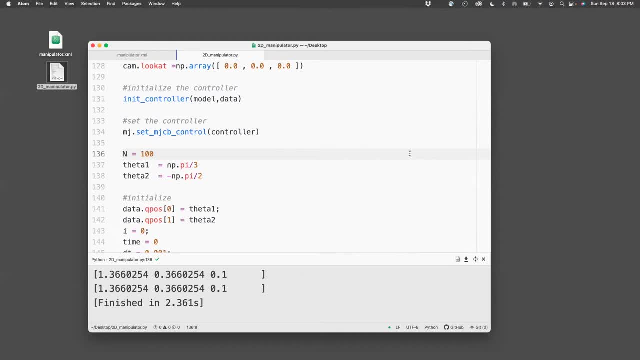 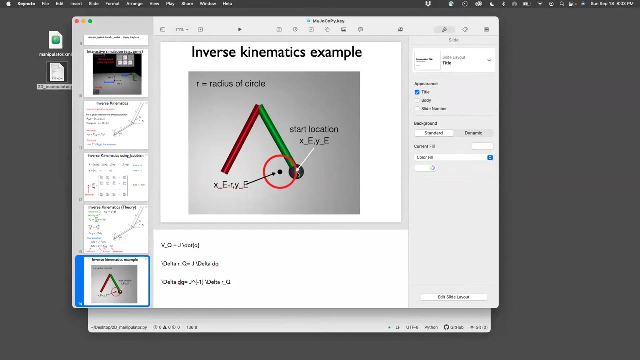 Now here. I don't quite have it at the end, the exact location I showed in the PDF- But it's OK, We can start from that position to draw the circle Now. what I'm going to do next is the following, which is: 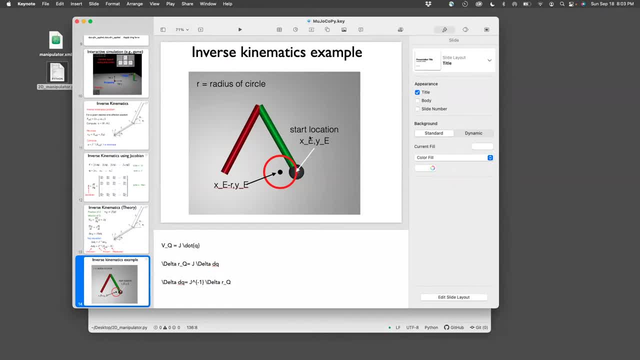 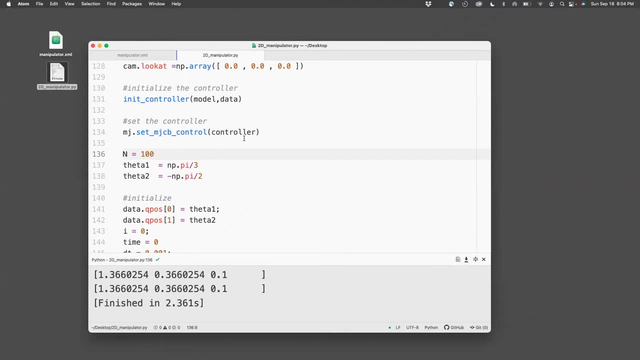 since this position is not exactly on the x-axis, it's somewhere here, I will first try to get the position of the end effector. To do that. I can access the end effector position right here By first running a forward step. 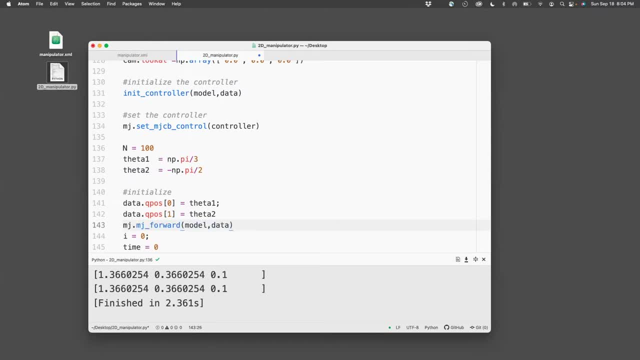 so forward kinematics, in this case that passes the model and data, And then I can read off the position of, in this case, q, which is the end effector as datasiteexpose, So that site is specified in here. 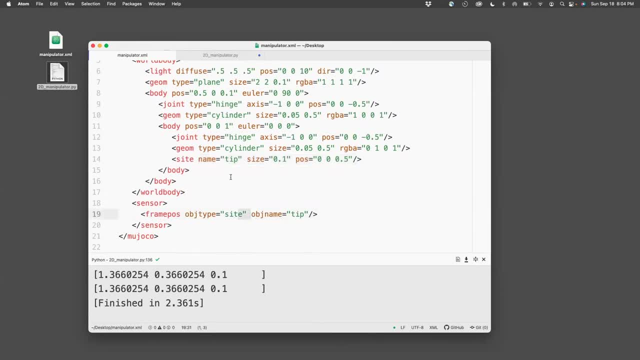 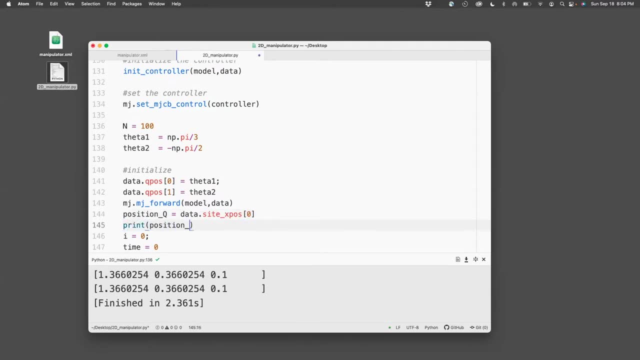 And since there's only one site, I can access that by passing on index 0.. So if you want to see what it looks like, just to print position q and run this, And it seems like it's printing something else in the loop. 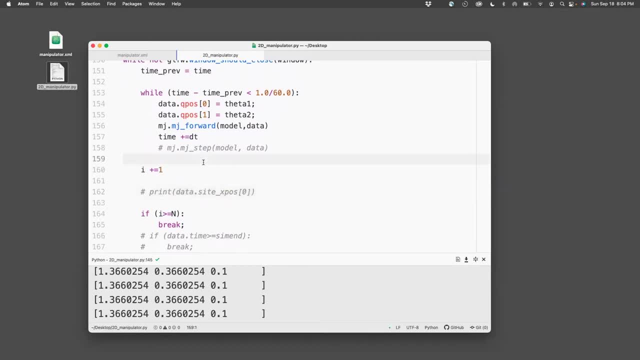 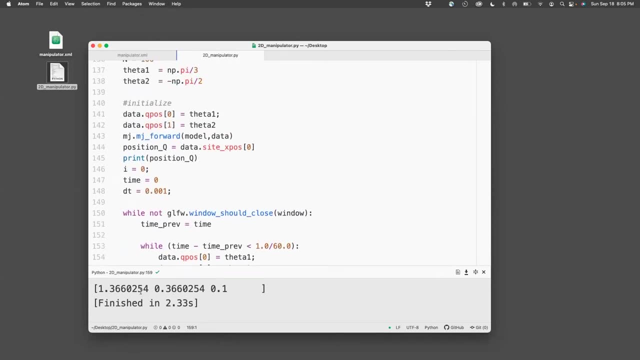 We can comment this out and rerun this again. So now it's just printing it once, which means it's printing this. So this is the position of the end effect. So what I'm going to do now is pretty much use this end effective position to specify the center. 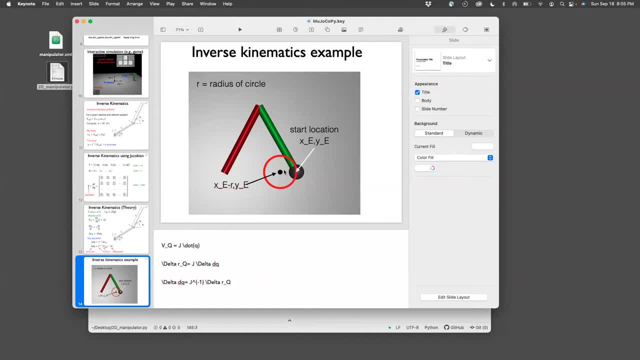 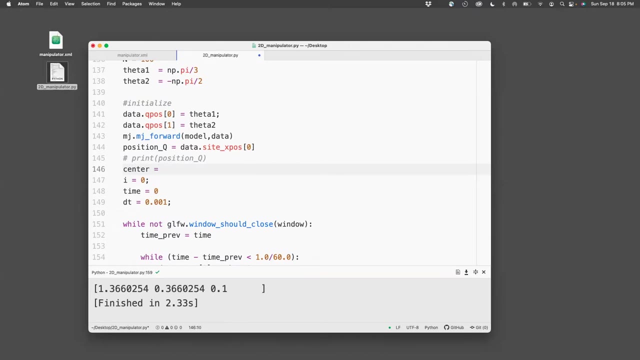 So if this is the end effect, if this is the start position, then the location of the center is going to be xc minus r ye. So that's what I'm going to do now. So the center equals npray Position q 0, that's the x value and minus r. 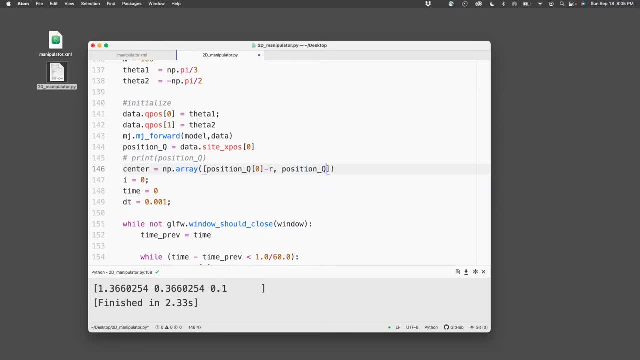 which I need to specify what r is and position q 1.. And let's choose r radius to be, let's say, 0.1.. So this gives me the center And now, since I have the center and radius, 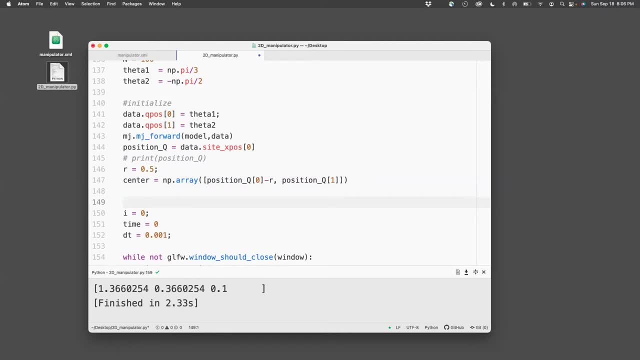 all I'm going to do now is I'm going to specify my reference. The way I specify the reference is: I'll define a variable field which wraps around the circle. so len space 0, times nppy n And my x ref now is going to be center 0, plus r times npcos phi. 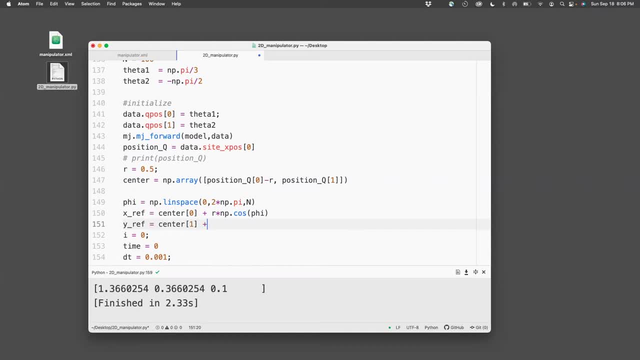 And my y ref is going to be center 1. Plus r times npsin p, And this basically coordinates along the circumference of the circle starting from the point I showed earlier in the notes. So now we have the reference, We can now start playing with the loop. 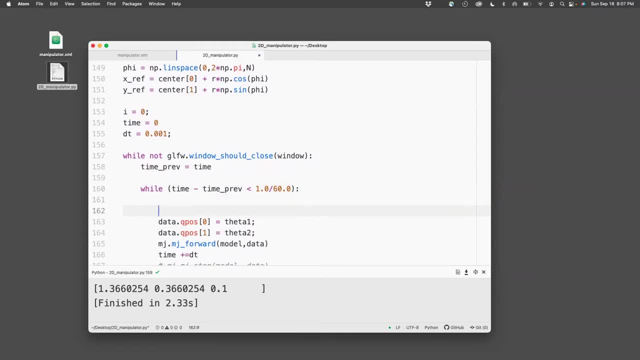 What I need to do is the following: I need to get so compute japhobian j. I need to compute. I need to compute inverse japhobian j- inverse- I need to compute the correction. So dq will be j inverse times dx. 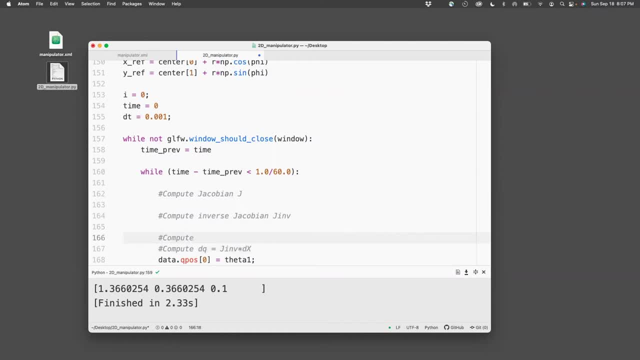 And since I also need dx, I need to compute dx, And once I have computed dq, what I would do is update: OK, OK. So let's see how these steps are done. So let's first compute the japhobian. 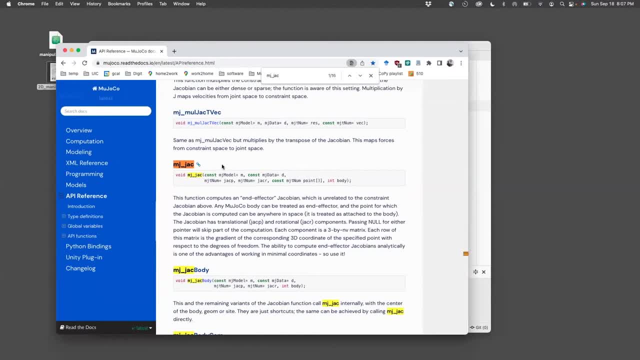 For that I need to look at the API reference. the API reference: I search for mj underscore jack. This command will give me, or this function would give me, the japhobian. You need to pass the model data. Jack P is the japhobian associate with the xy motion, xyz motion. 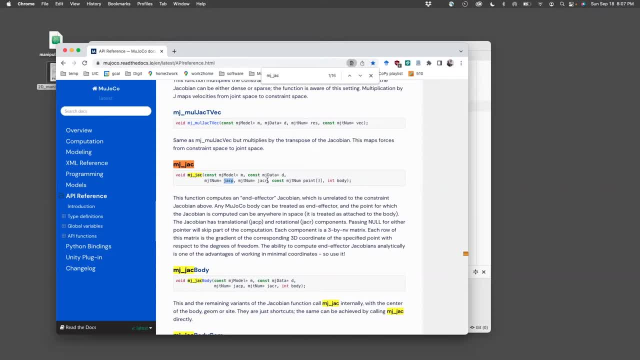 Jack R is the japhobian associate. There we go is with the rotation of the end effector. We do not have to worry about this in this particular case, because we are not looking at rotations. We need to pass the point. 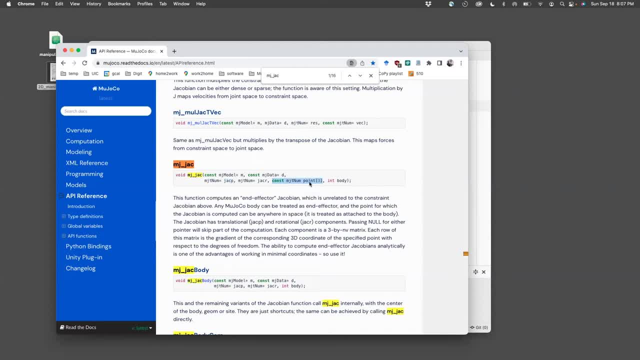 In this case, the point is the position of E, the end effector, And then we need to specify which body it is. OK, so let's do all these things. I'm going to copy this And note that this is not Python code. 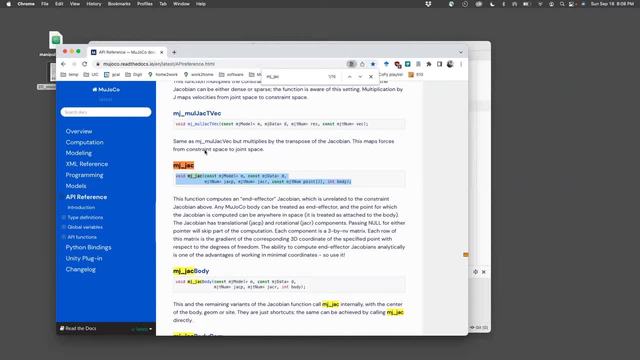 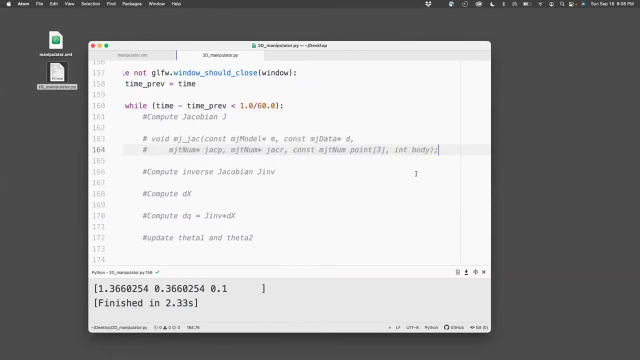 but this is actually the C function, But we need to interpret it appropriately in Python. So let's put it here. Let's see how to go about doing this. So we say mjmjjack, We pass the model theta, Then we have jack p. 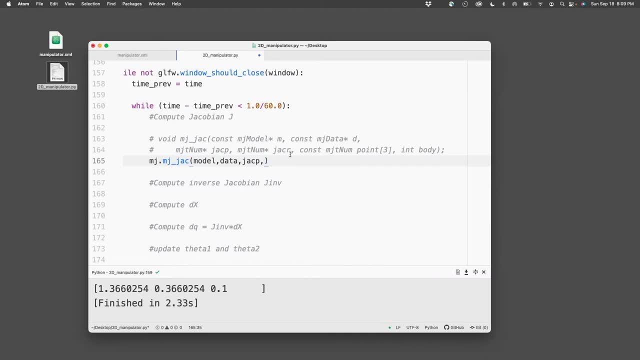 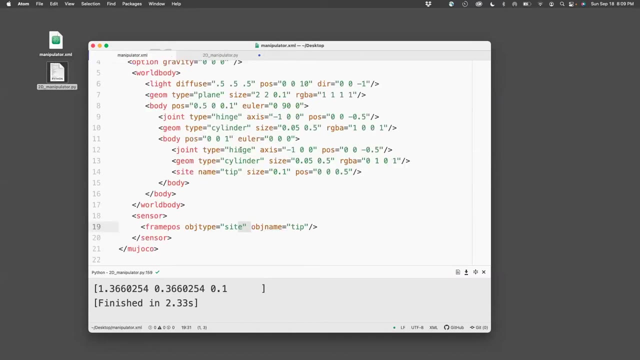 Then we do not quite need the Jacobian with respect to the rotation, so we can pass none. We need to pass the position of E And then we have to compute the body. Now, if you look at this, you can find the body number. 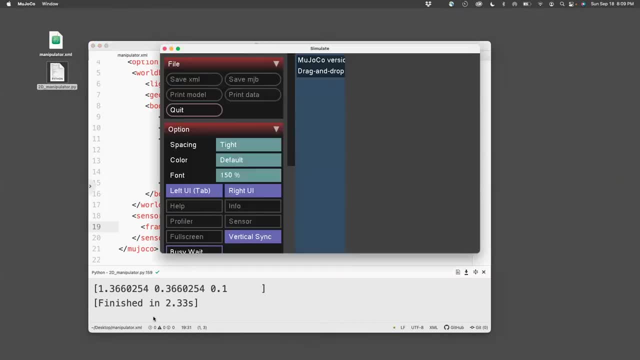 over here. Or another way of doing it is to open, go to the simulator, drop the XML, say print model, then locate where the simulatorexe is And that model will tell you. the print model, which will be mjmodeltxt, will tell you the body number. 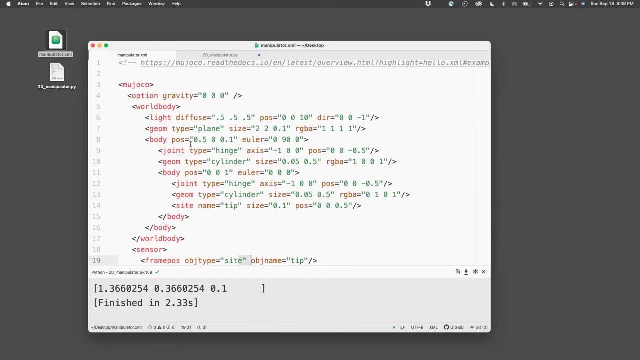 for the last link. Now, in this case it's kind of easy to compute that number: The world body is always body 0. The first link is going to be body 1. And the second link is going to be body 2.. 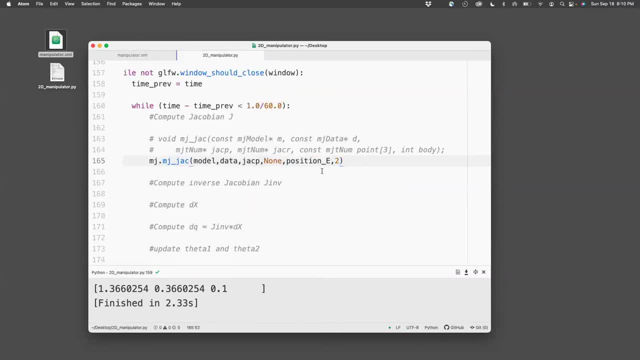 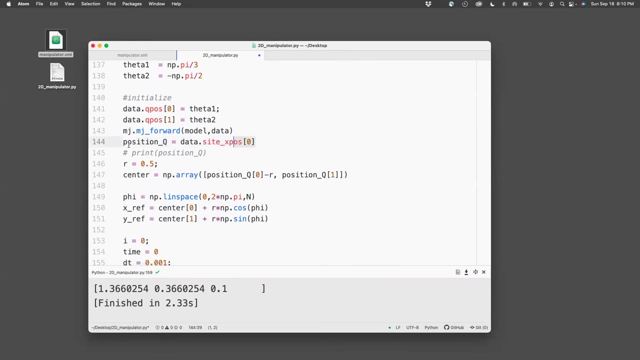 So we need to put number 2 here, OK, So now we have this. Before we do this, let's try to get what position of E is So? position of E. we actually did this step here. Position of: oh sorry, I said Q, So let's. 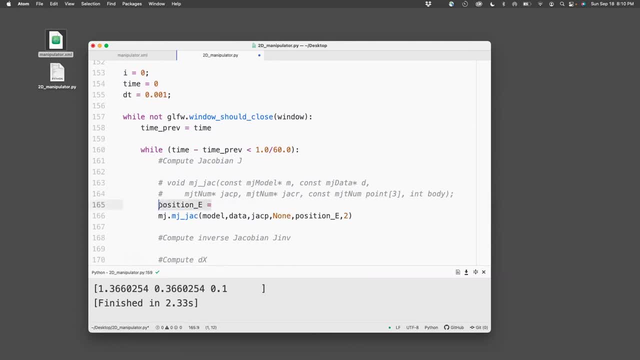 call that position of Q. So I'm going to change this name to Q, which is to be consistent. So that's specified. The Jacobian is: remember that we're trying to compute the Jacobian of the end vector, which is going to have x, y, z coordinates. 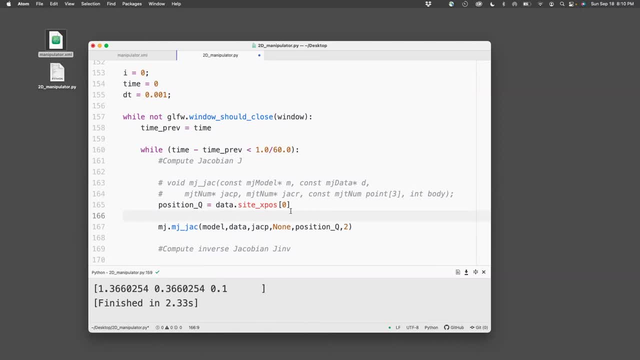 And that Jacobian is with respect to theta 1 and theta 2.. So the size of P, we need to initialize this, So I'll say np.0s, 3,, 2.. So the 3 is for x, y, z. 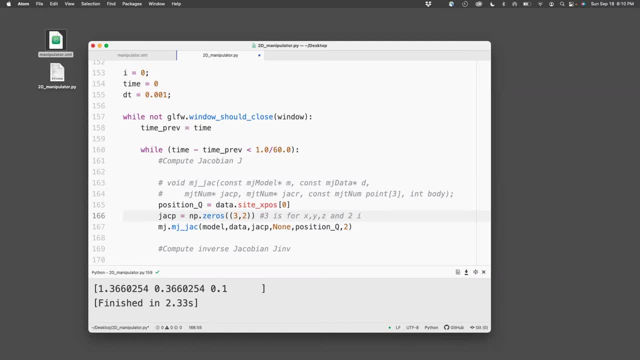 And the 2 is for theta 1 and theta 2.. So we specified this for Jack P, position Q, And now we're going to do the same thing for the second row. So we're going to do the same thing for the third row. 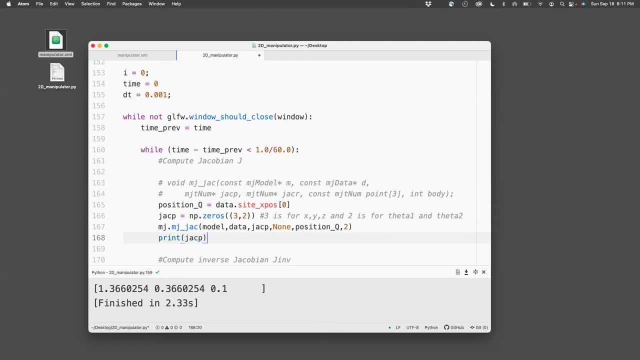 And now let's see what it will give us. So print Jack P And note that this is going to run in a loop. So we'll keep printing this again, but for the same position. So it's printing It stopped. 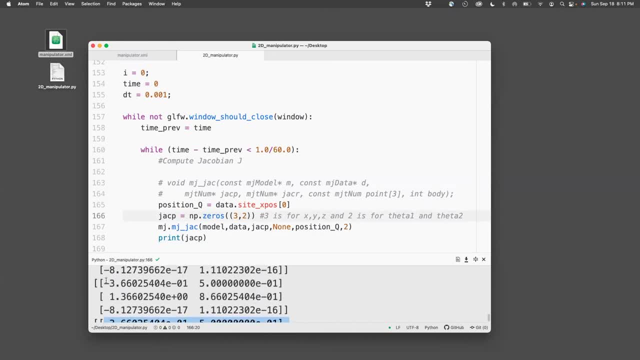 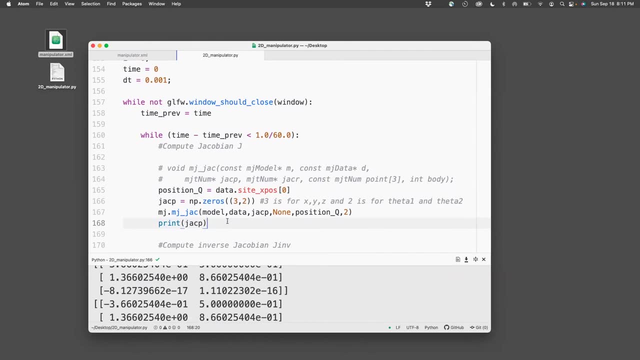 So this is what it looks like: 3 cross 2.. We'll have the same value here, and so on. So what we need to do here is: we don't need the third row, Because we're only interested in Jacobian of x, y, with respect. 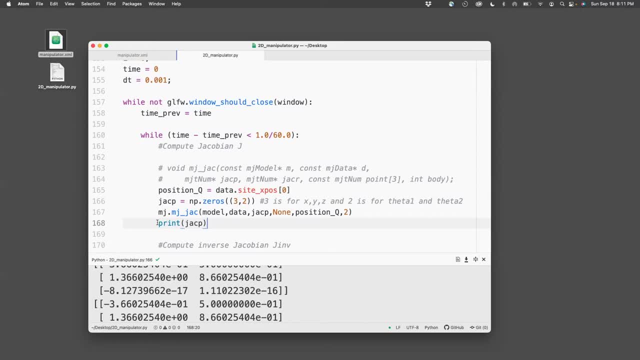 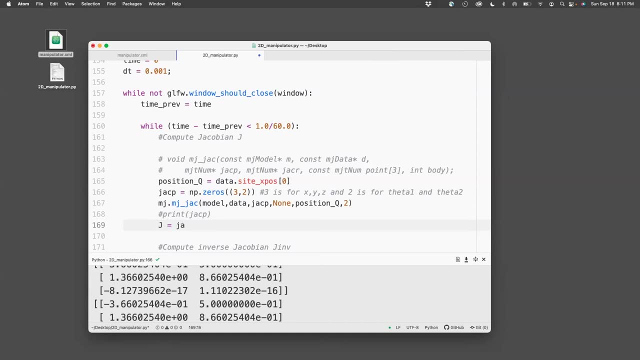 to theta 1, theta 2.. And we don't want the z-position. So what we'll do is we'll define J to be Jack P And we only take the 0th and 1st. That means the first two rows and all the columns. 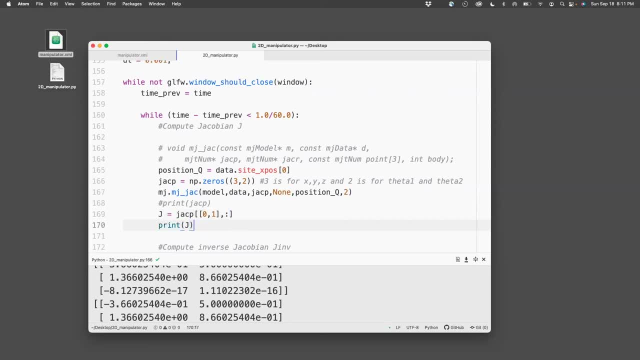 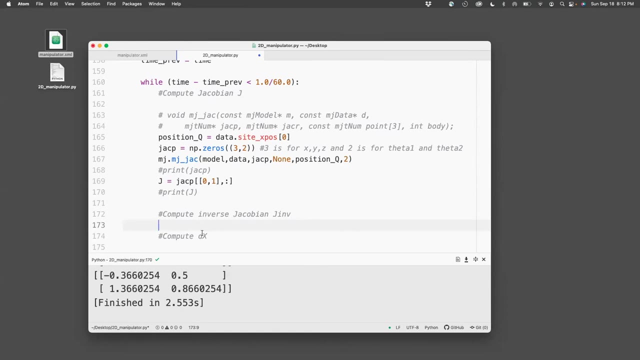 And so if you want to check this again, you print J And then you can see it's printed 2 comma 2.. Now that you've got J, we can compute the inverse. The inverse is available in LIN-ALG. 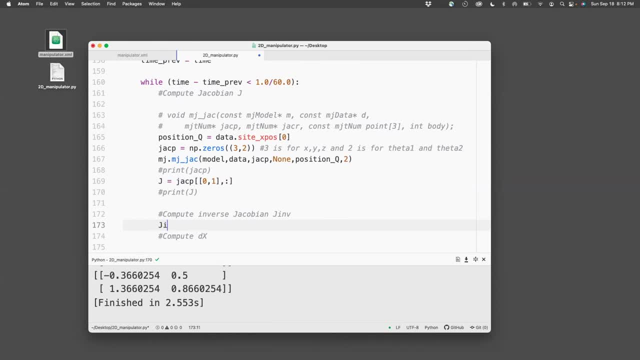 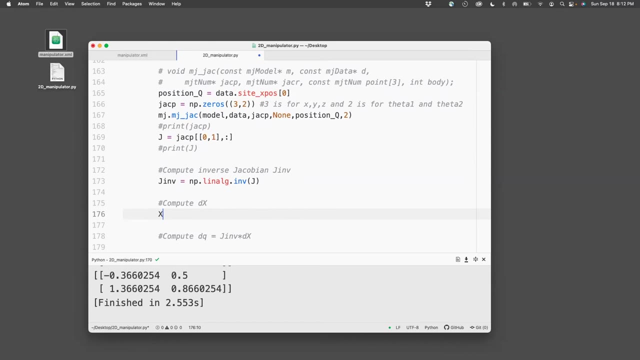 So it is J inverse equals NP dot LIN-ALG dot inverse J. That will give me J inverse. Then I need to compute dx. So dx is x ref minus x. So what's x ref? x ref is the reference position. 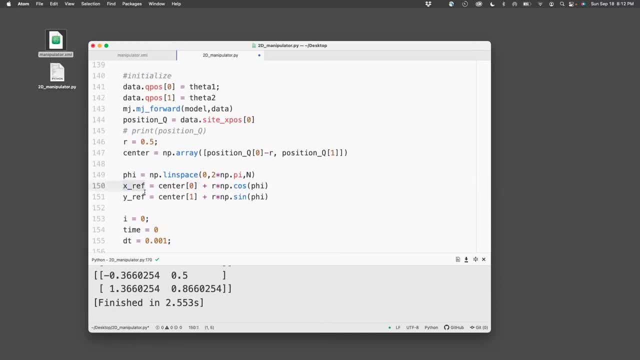 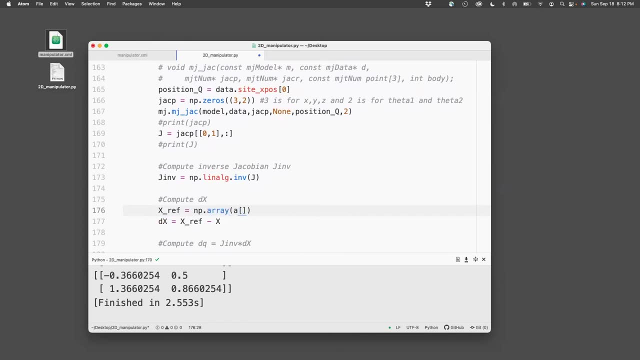 This is something which I already specified here. I just need to pack that in an array. So I'll pack that as numpy NP dot array. Position q 0.. Position q: 1.. And x is my reference position. x is my sorry, this should be. this should be. this is actually the measured position. 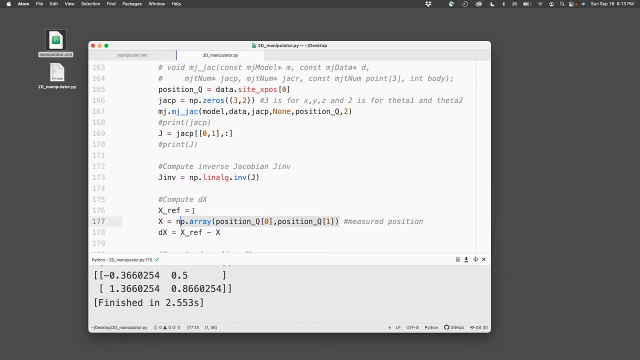 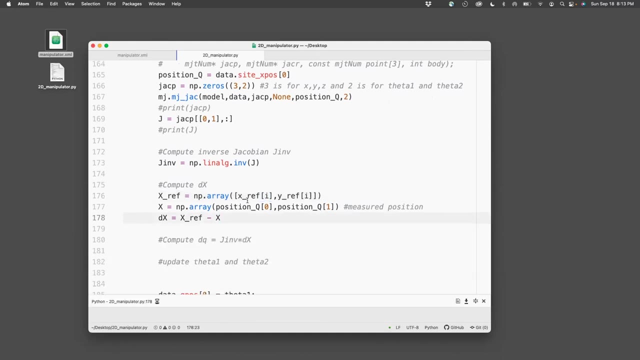 And this should be the first one should be the x ref, NP dot array, x ref, y ref And this should be index i. Let's see if this runs fine. Okay, It runs fine. Didn't print anything, It's fine. 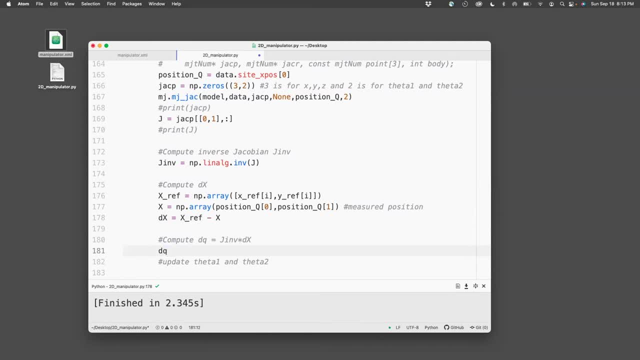 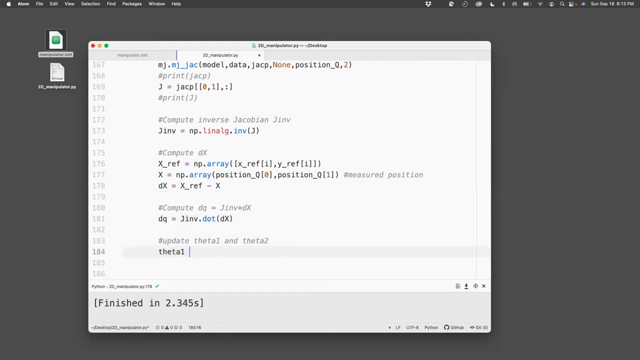 Okay, Now I can compute dq. dq is equal to J inverse dot dx. This is just doing the multiplication of a matrix times the vector. And now, once we have dq, we do: theta 1 plus equals dq 0.. And theta 2 plus equals dq 0.. 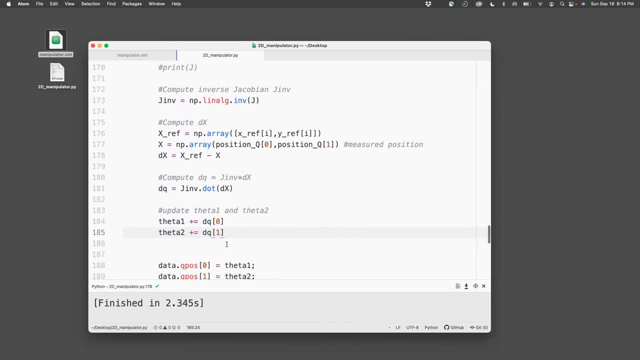 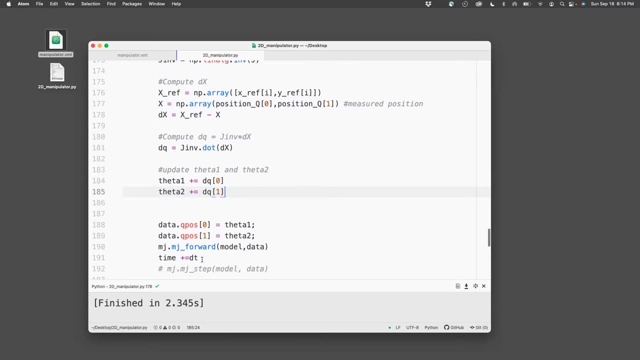 So we've updated it, Then it goes into it- updates in the data variable of Mojoko, And then we do a forward step increment time and nothing needs to be changed here. So let's just run this. Okay, So it didn't look like it worked. 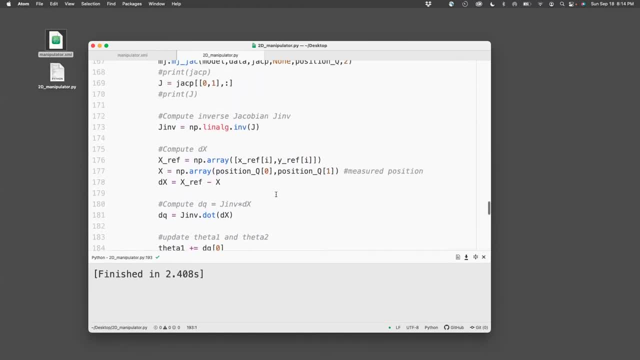 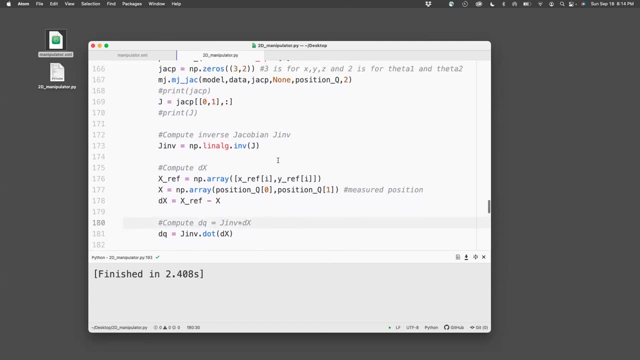 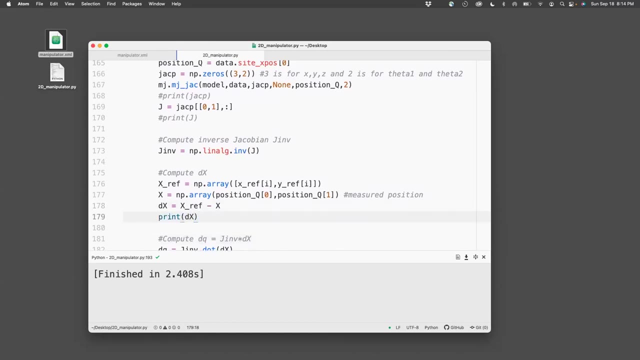 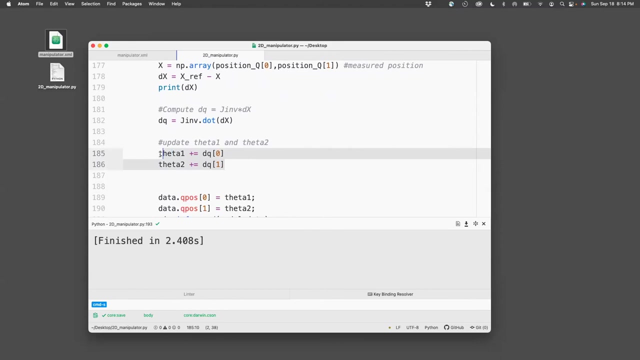 We'll try to debug this. Okay, Perhaps let's try to see if we can print something. So print the x. Let's not do this update because it gives me it's, it's, it's, it gives a problem. 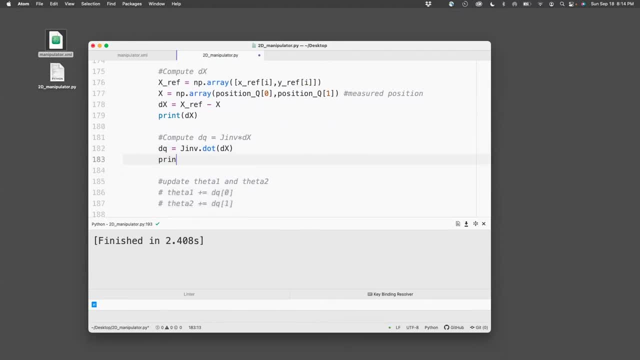 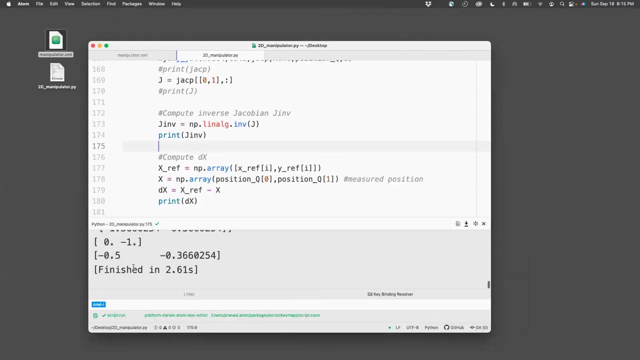 So it just keeps moving. Let's try to print dq And let's see what's going on there. And also let's print J, inverse, Okay. So if you see this, let's see, So we have. this is dq. 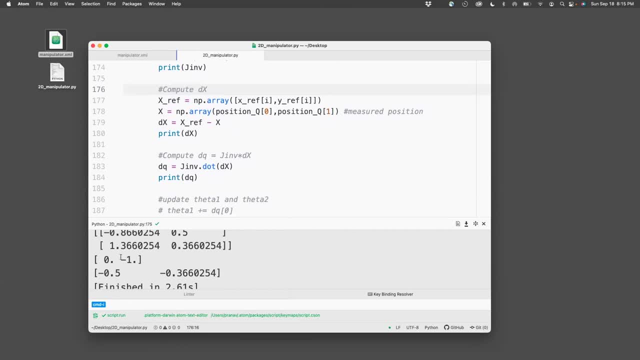 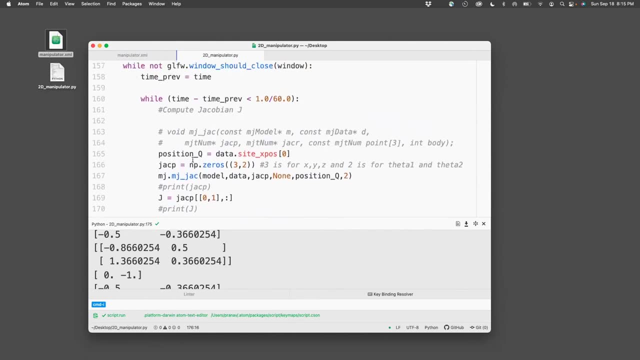 Looks pretty big. This is dx. This also looks big, And then we have J inverse, So nothing really looks wrong here. Let's see if we can understand if we did some errors somewhere in the code here. So position of q is correct. 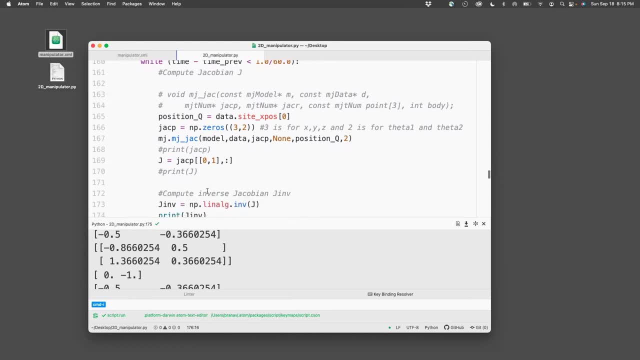 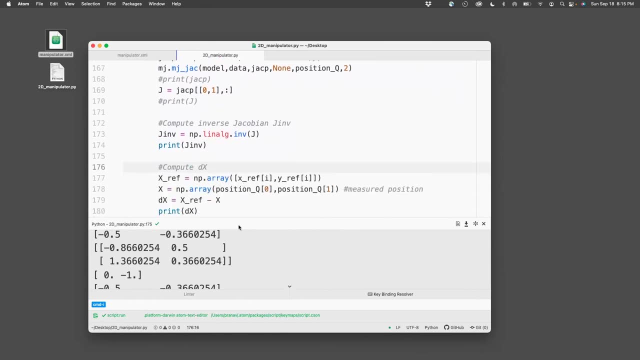 Jackp looks good, J inverse looks good, X ref is good. Okay, I think that this does not work the way it should work. So it should be dx equals- Okay, I think that this does not work the way it should work. 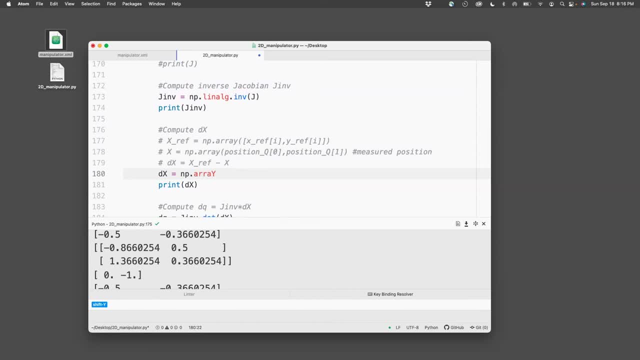 So it should be: x equals np dot array, X ref minus position q zero And y ref minus position q one. Okay, Because this subtraction doesn't really work the way I do this, I've specified it, So let's see if this works. 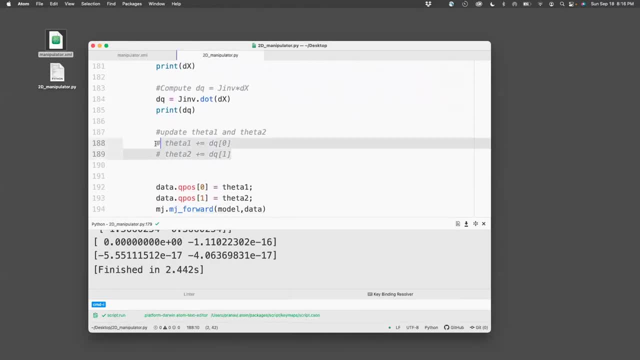 Okay, So I need to re-enable this update. Let's run this. That worked. Okay, So the error was in this part of the code. This is not the right way of computing the difference, So let me just delete this part.